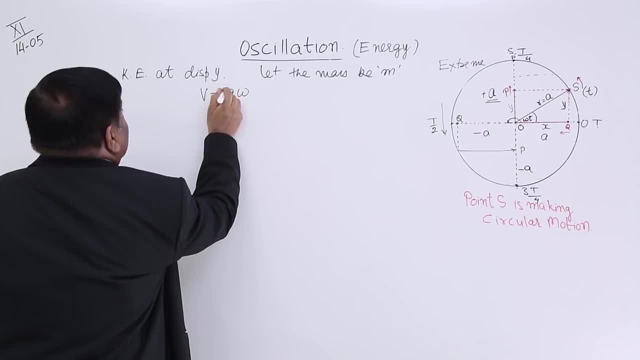 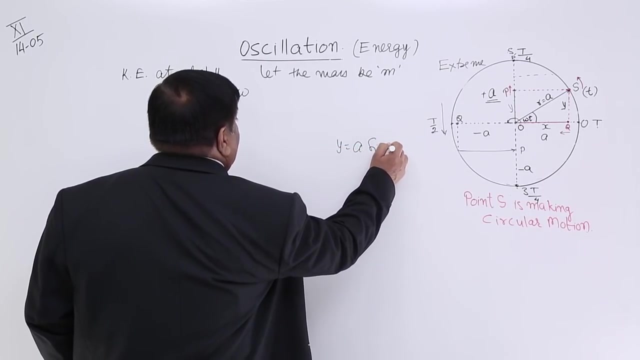 a omega plus minus. Okay, a omega is maximum velocity. You know the equation of displacement was: y is equal to a sin omega t, And the displacement dy by velocity, dy by dt was a omega cos omega t. So the velocity is a omega. 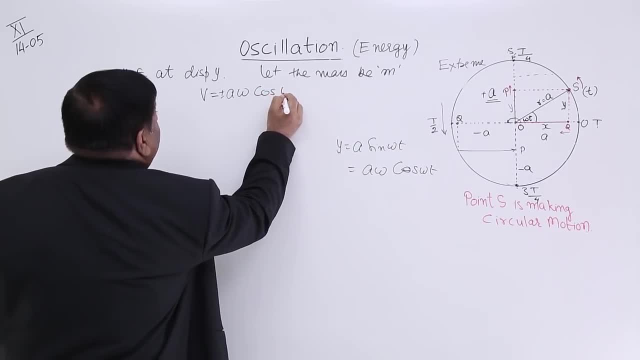 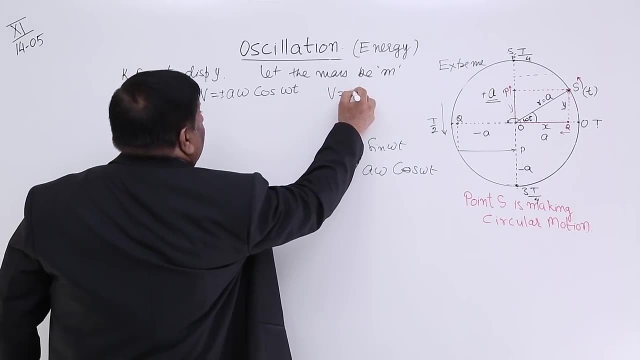 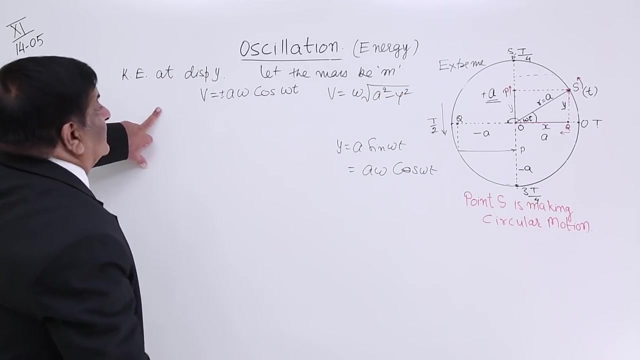 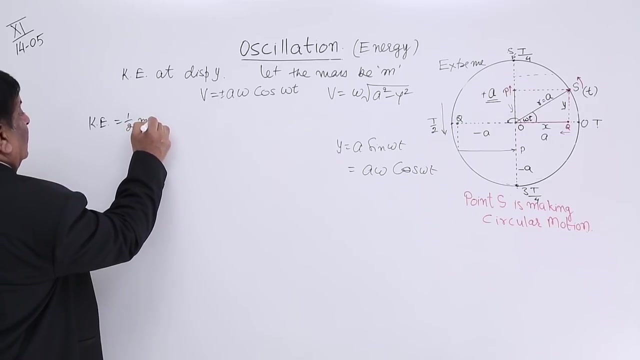 So the velocity is a omega cos omega t And in the terms of y, this velocity, we wrote a formula omega a square minus y square. So when I make convert it into energy formula, that is half mv square, Kinetic energy equal to half mv square. 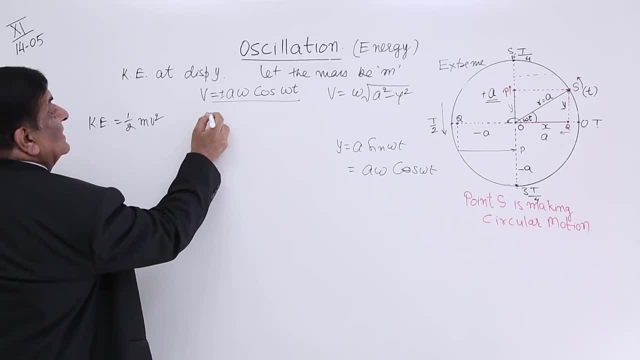 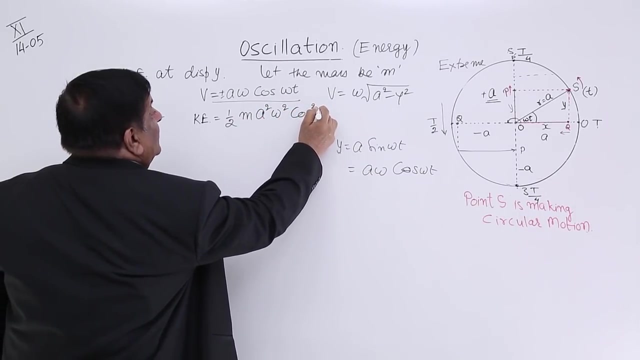 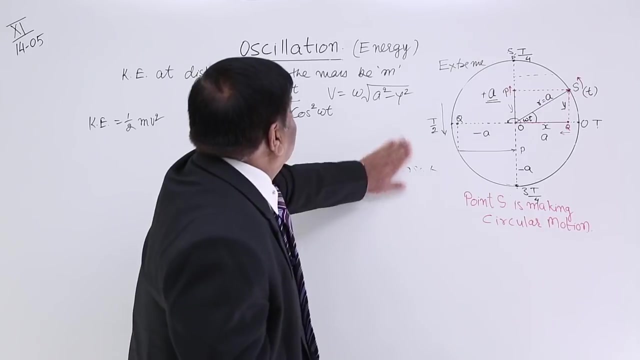 Then, using this velocity formula, we get kinetic energy. Kinetic energy is equal to half m into square of v. Square of v is a square omega, square cos, square omega t. When I use this formula, then we get this equation as kinetic energy. 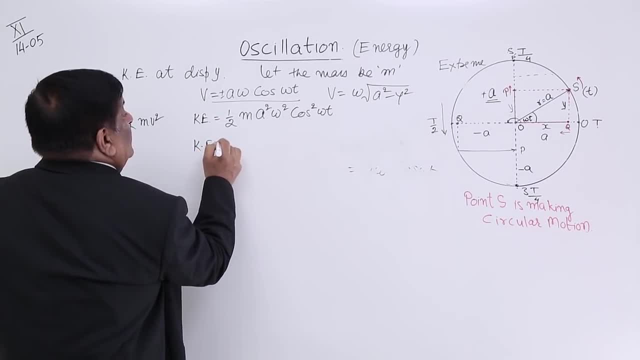 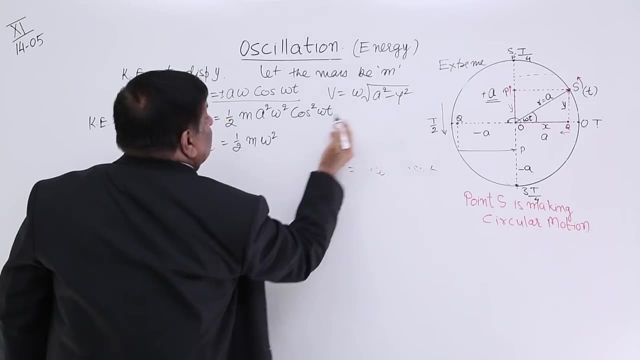 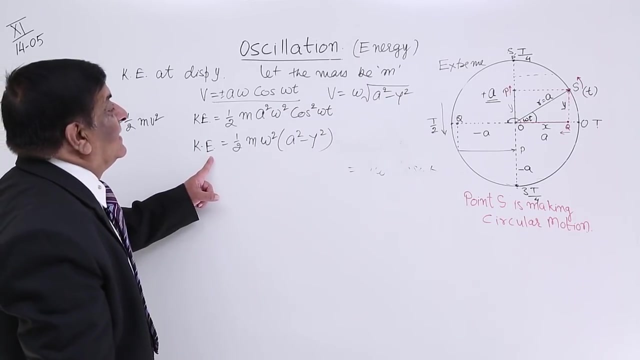 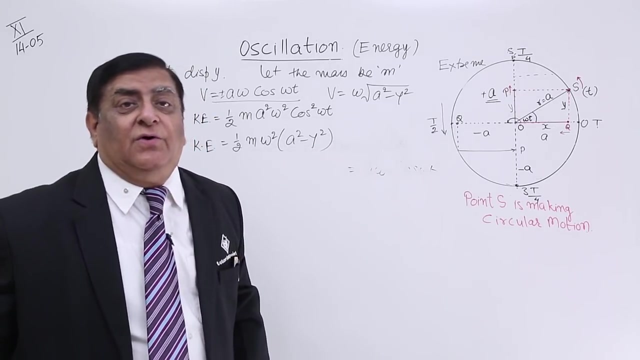 Ke is equal to half mv square, omega square, and square of this is a square minus y square. So we have two relations of kinetic energy, One at time, t, one at displacement, y. So this is how we have two equations of kinetic energy. 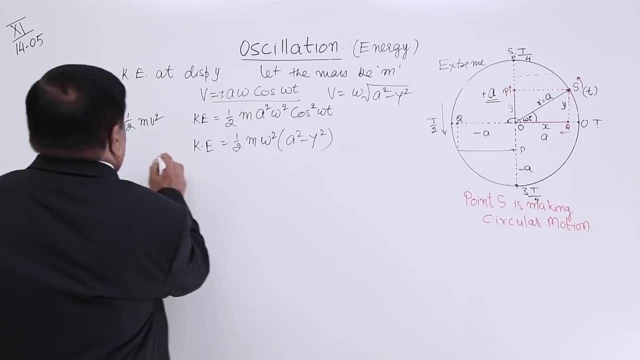 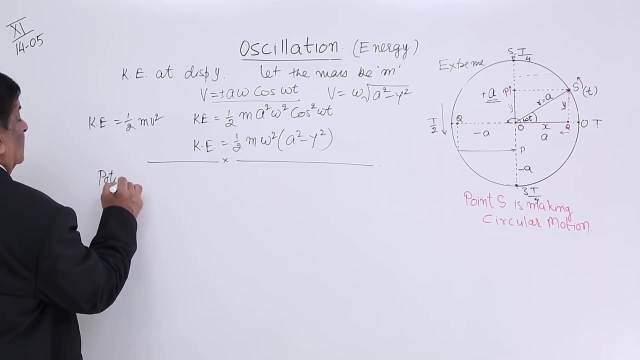 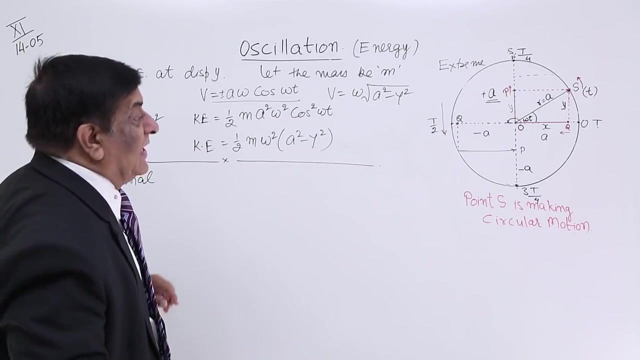 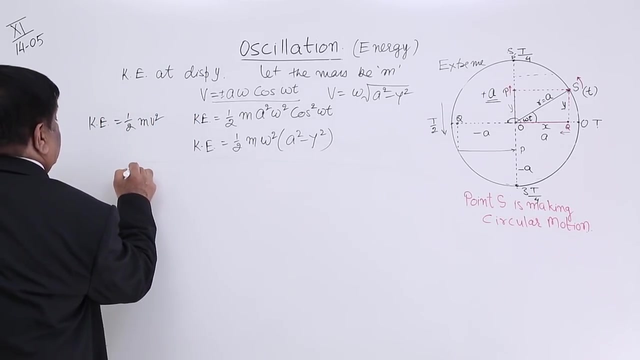 When the displacement is y, How much should be the potential energy? Or another thing here: What is the maximum kinetic energy and where is the maximum kinetic energy? So maximum kinetic energy When this minus portion is zero? So if it is zero, then what is the amount of maximum kinetic energy? 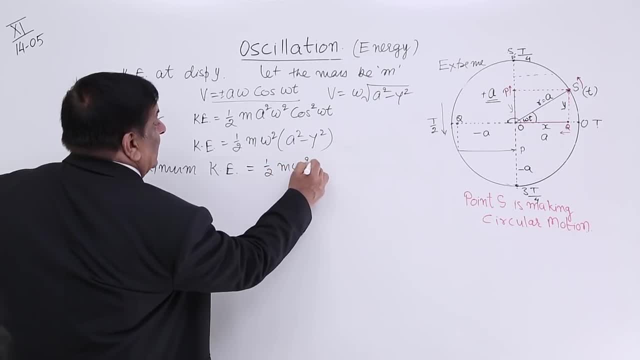 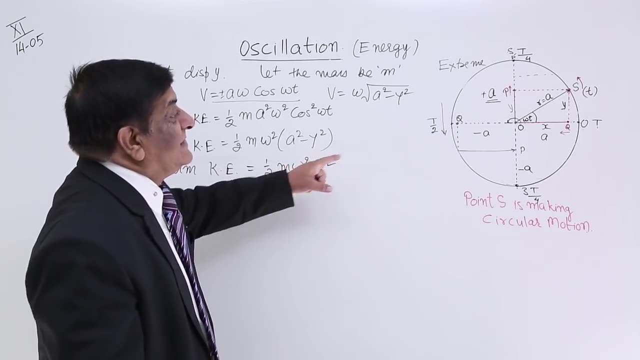 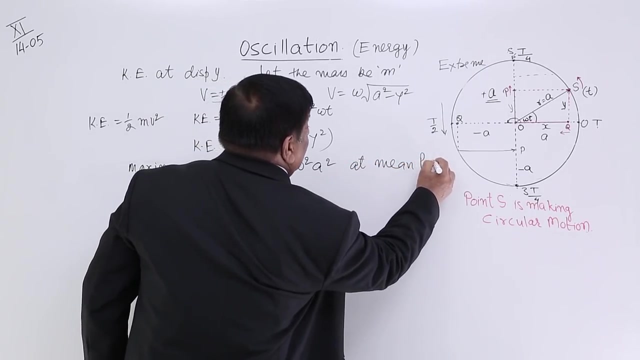 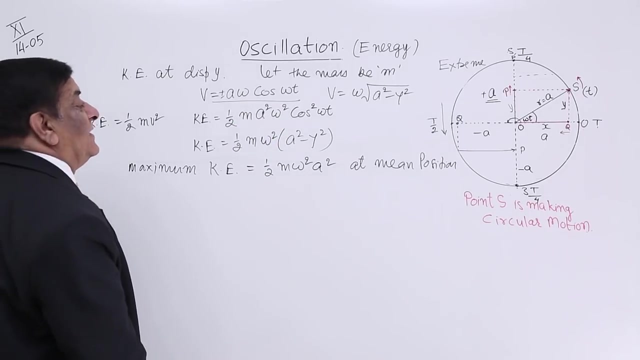 That is half m, omega, square, a square. This is maximum kinetic energy, And where it is, Where y is equal to zero And where y is equal to zero At mean position, At mean, So, at mean position, kinetic energy is maximum, of course, because velocity is maximum there. 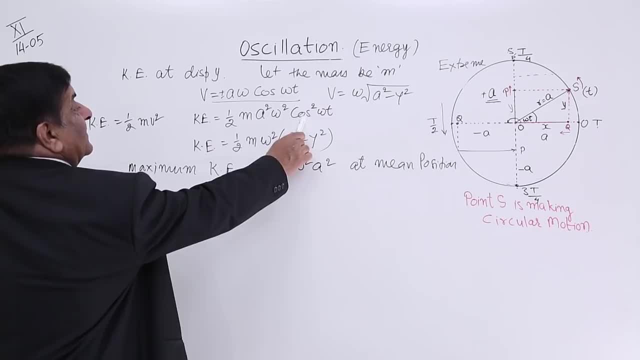 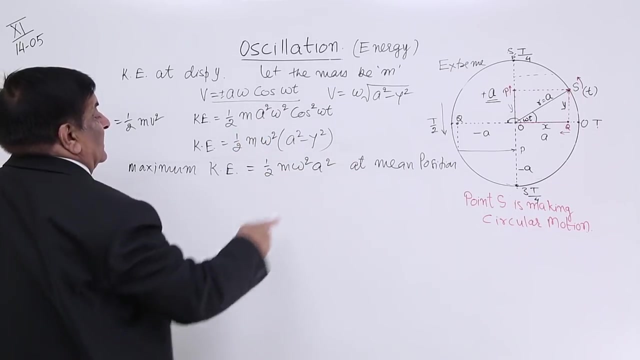 Right, If we put here, the maximum value of cos, omega t is equal to one. Put one here. What do we get? Half m a square omega, square, Half m a square omega. So either by this or by this You get maximum energy. 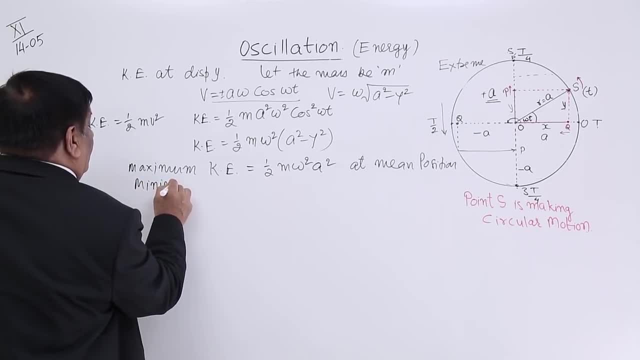 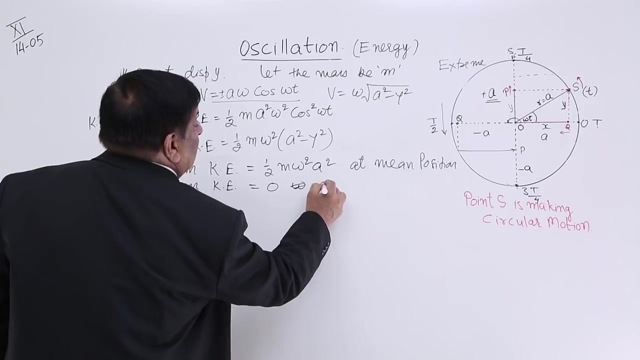 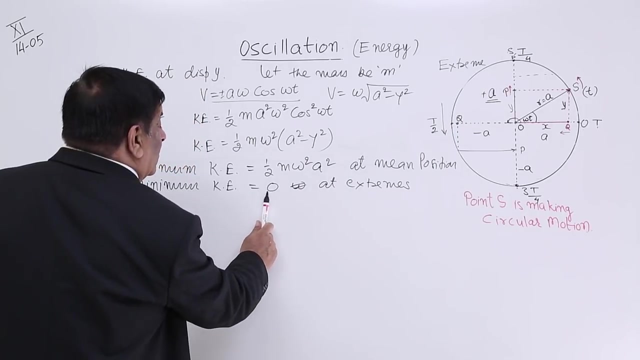 And where this is minimum, Minimum kinetic energy, Minimum kinetic energy, Minimum kinetic energy. where velocity is zero, This is equal to a, So this becomes zero. So zero Where it is At extremes. So at extremes, kinetic energy is zero. 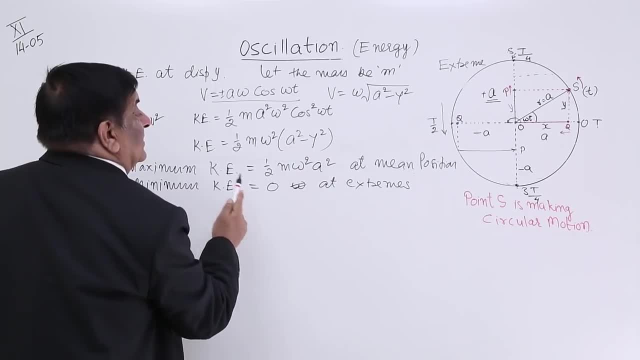 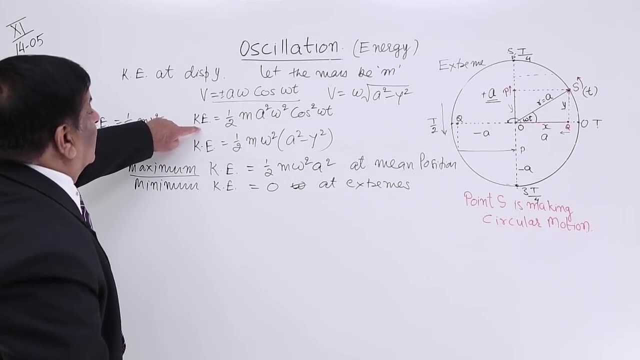 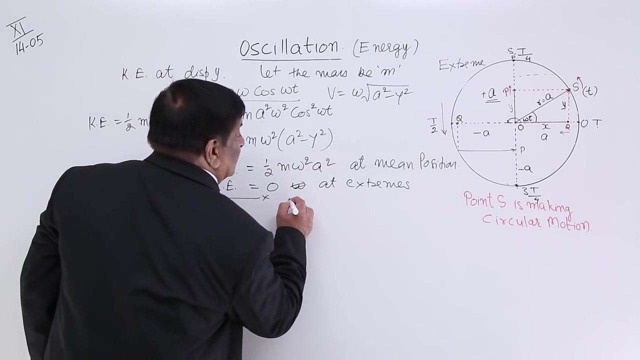 At mean position, kinetic energy is maximum. So this is special conditions of kinetic energy. So this is special conditions of kinetic energy. These are general equations of kinetic energy. This is maximum value of kinetic energy, And now we go for potential energy. 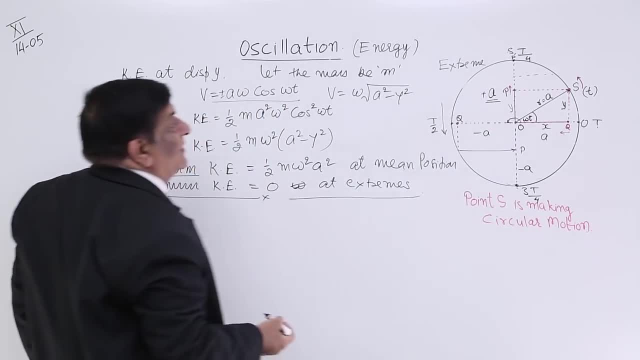 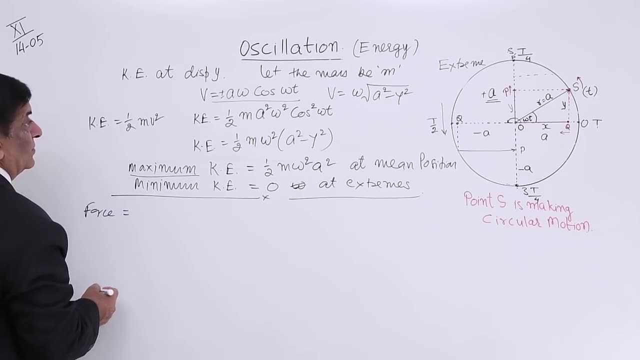 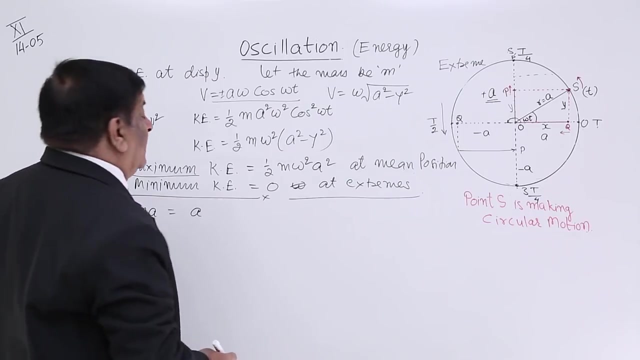 Here, at any displacement, y, how much is the force? Force is equal to mass into acceleration, That is, mass into. what was the equation of acceleration? That was y, omega, Y omega Minus y omega square. This was our equation for acceleration. 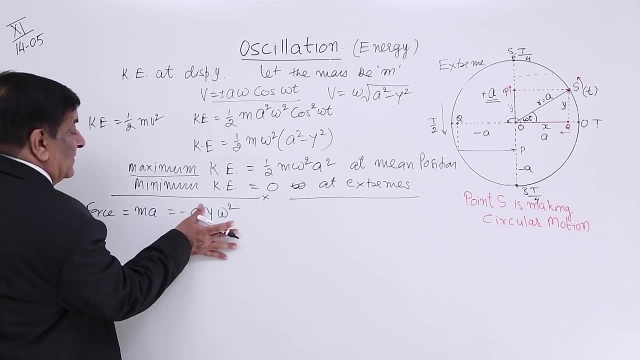 So if we multiply it with mass, Mass, Mass into acceleration, Mass into acceleration, This, We know the value of alpha. What was that? Minus y omega square. And this is the force acting on it. Now, if this is the force, then how much work has been done? 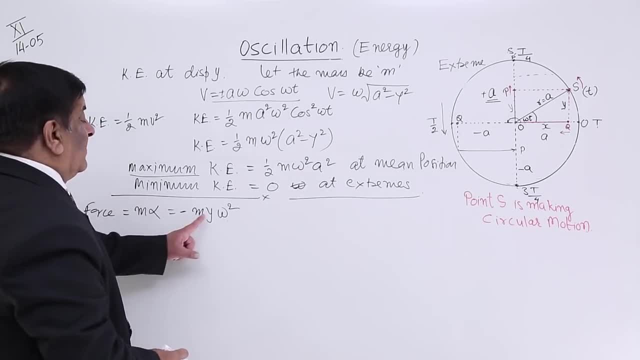 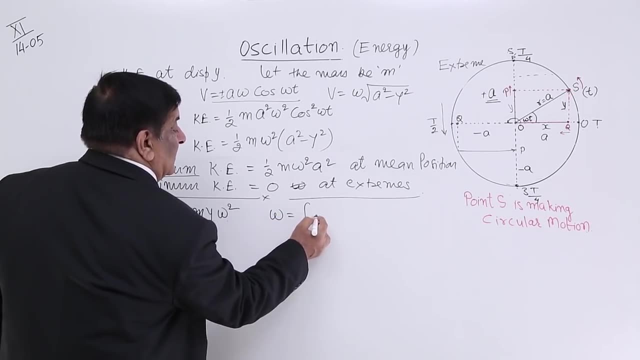 How do we find out? We know the equation for work is integration f dy Zero to y. If f is variable, then this is our calculation Force into displacement: Integration zero to y. This we have done earlier And here we apply it. 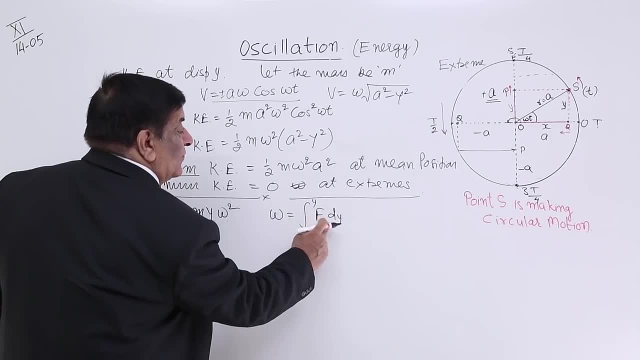 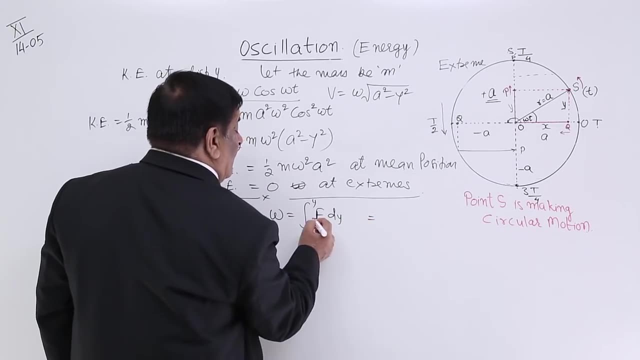 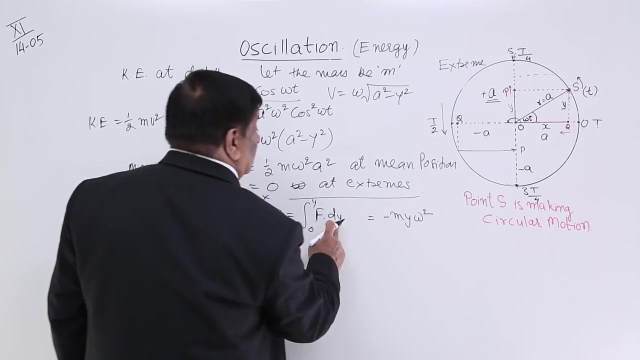 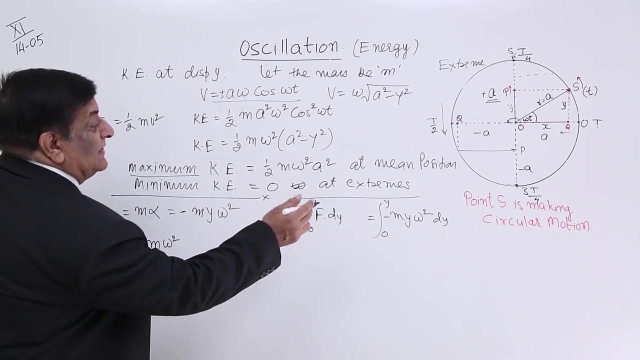 This is our calculation Force into displacement Integration zero to y. This we have done earlier, earlier, and here we apply it. Force is this: minus m y omega square and displacement dy integration 0 to y. So when we do it here it is m omega square, comes out y dy integration. 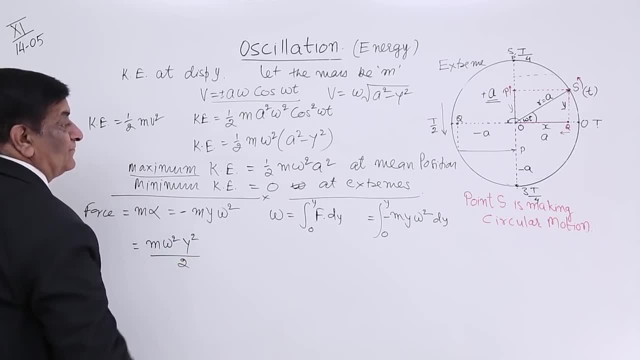 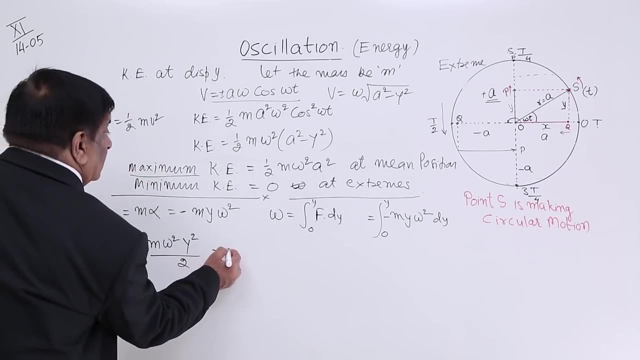 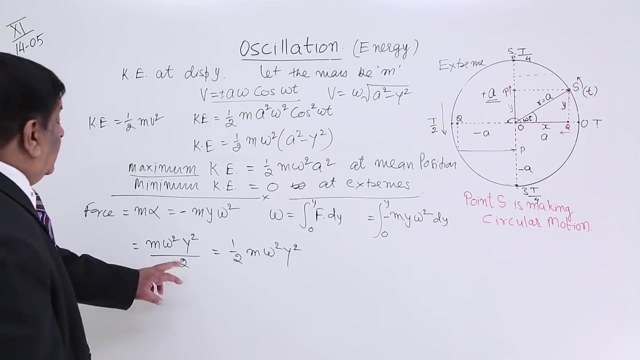 is y square upon 2. So this is equal to half m omega square, y square. So this minus we can reject, because this was telling only direction, So let us reject it. So how much is the potential energy? The potential energy is: 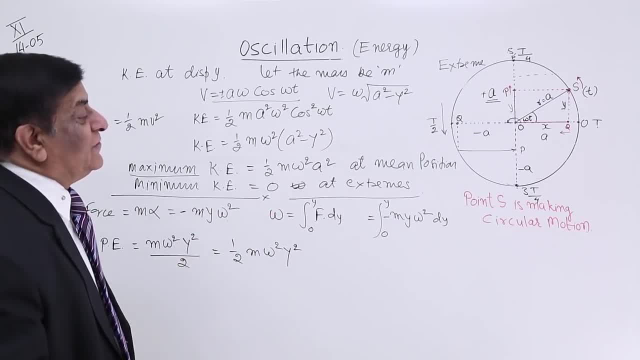 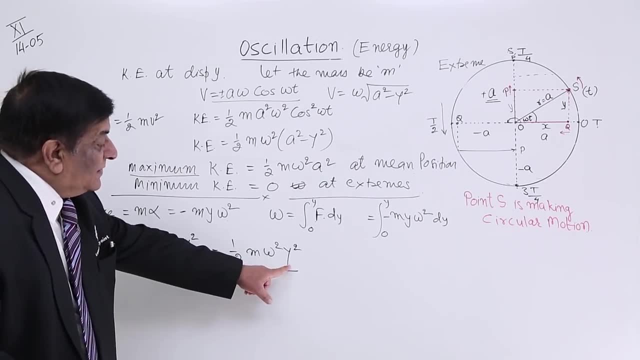 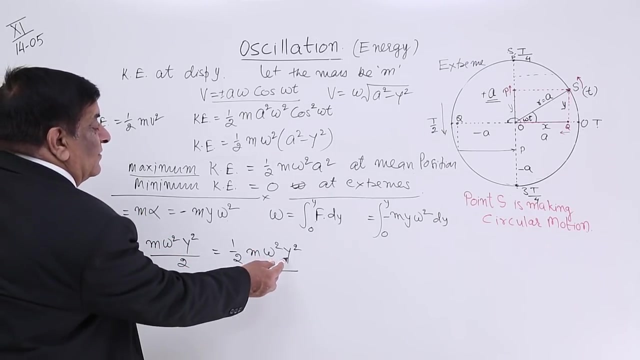 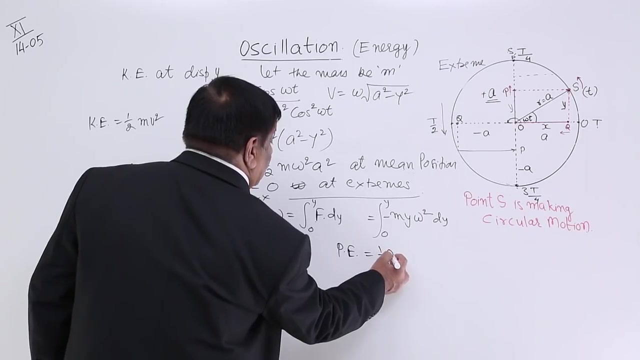 half m omega square, y square in magnitude right here. This is potential energy related to y. What is the equation of potential energy related to t? We can very well do: y is equal to a sin omega t. So we have another formula for potential energy that is equal to half. 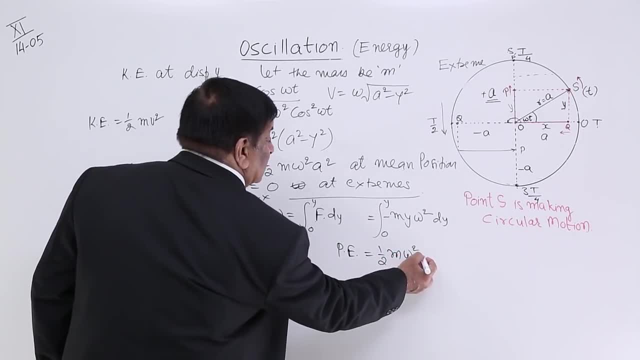 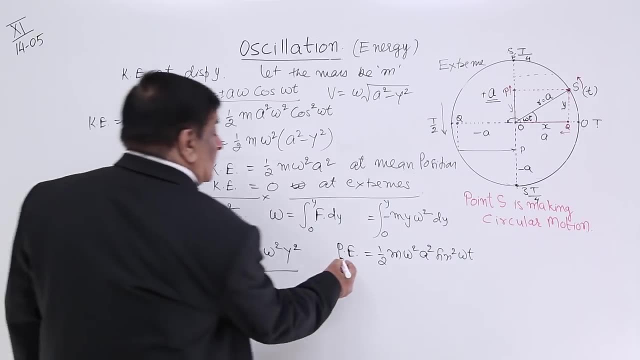 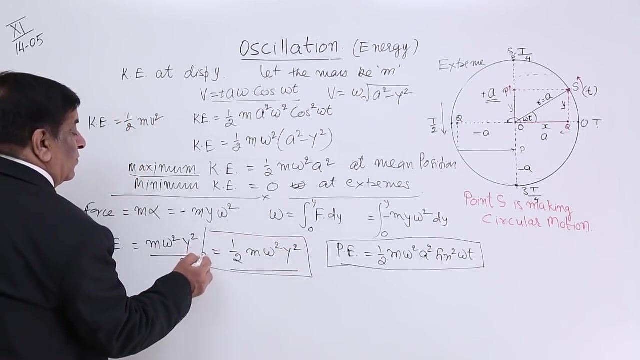 m omega square and y is equal to a sin omega t. So this is a square sin square omega t. This is potential energy at time t. This is potential energy at displacement y, Potential energy at displacement y. both are same thing. Now. 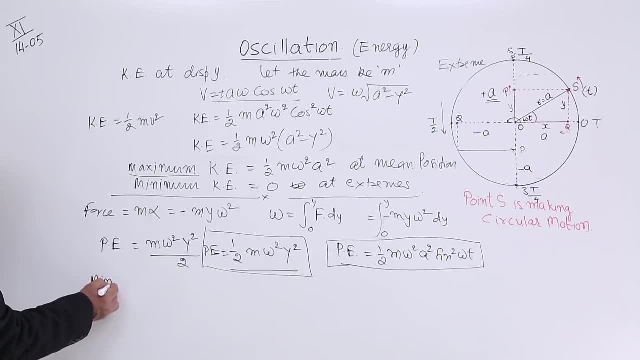 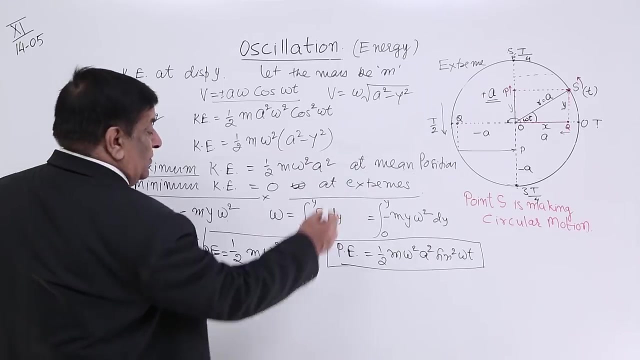 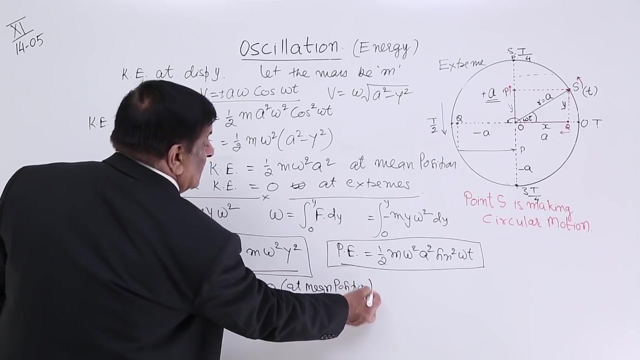 what should be the minimum. Minimum Pe is 0.. When it will be 0?? When it will be 0, it will be 0.. How much Level of energy? Level of energy be 0 when y is equal to 0, where y is equal to 0 at mean position? when it will be maximum? 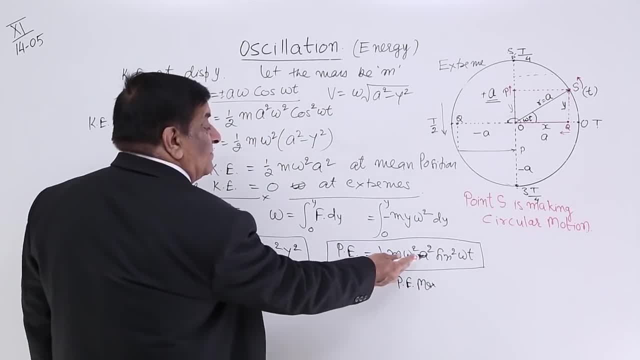 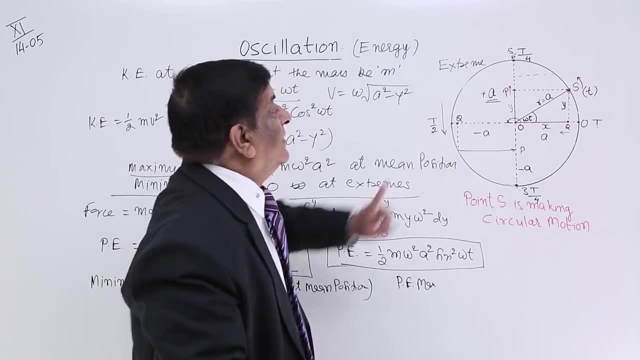 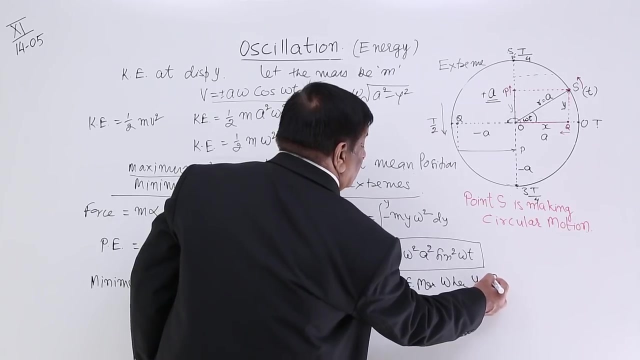 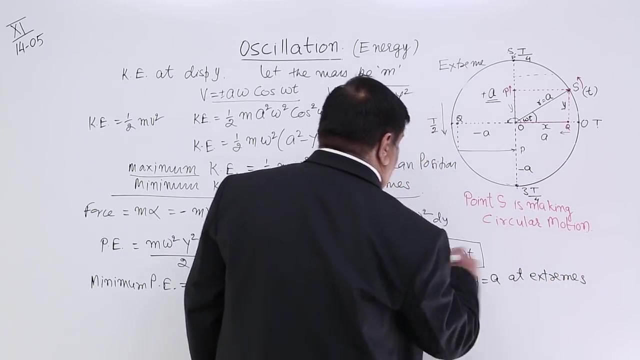 p e maximum, where it will be maximum when y is maximum. what is the maximum value of y that is equal to amplitude a. so p e maximum when y is equal to a. if y is equal to a potential energy is maximum. and where is this at extreme, at extremes, and how much is this? 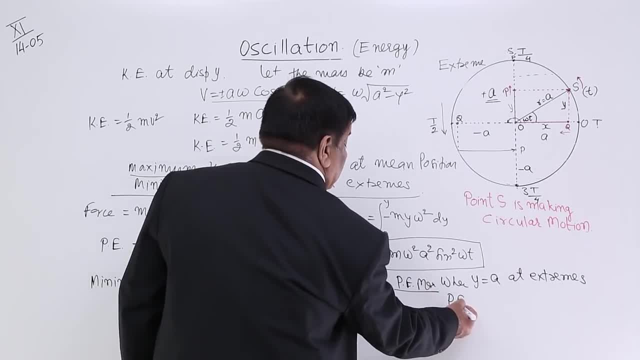 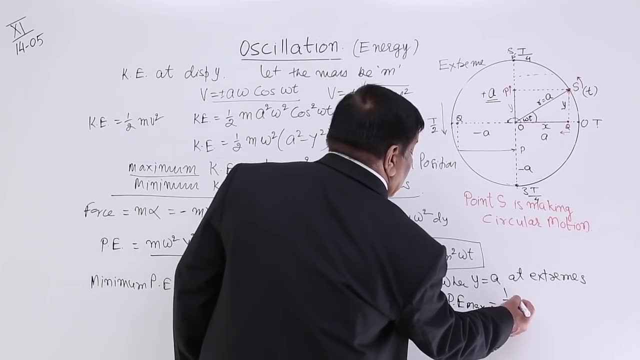 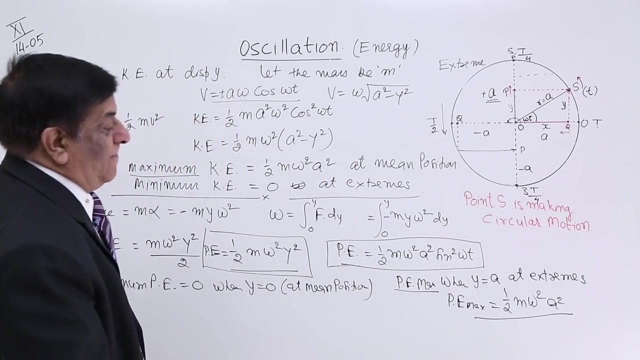 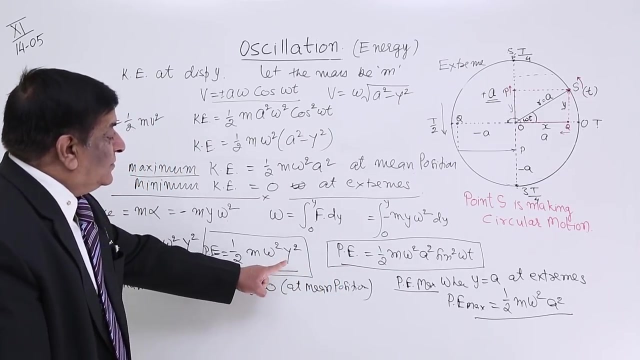 maximum potential energy. this p e maximum is equal to What y is equal to a, and we have here half m omega square, a square. this is maximum potential energy at the extreme. so this is general equation of potential energy. these two related. 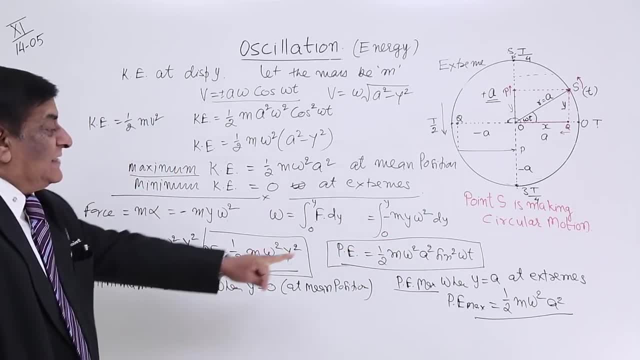 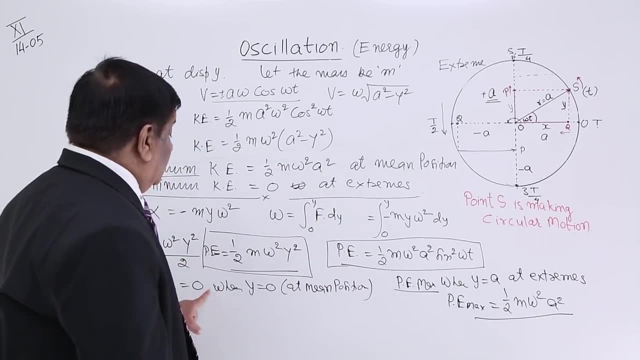 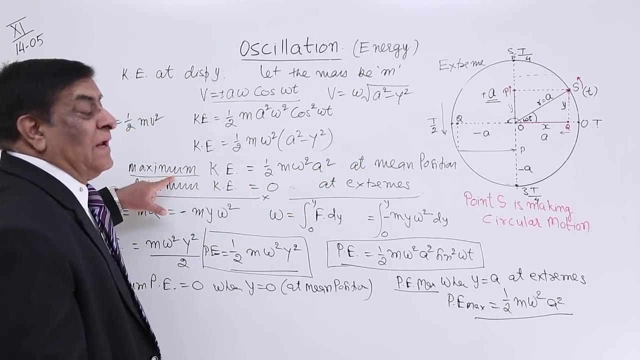 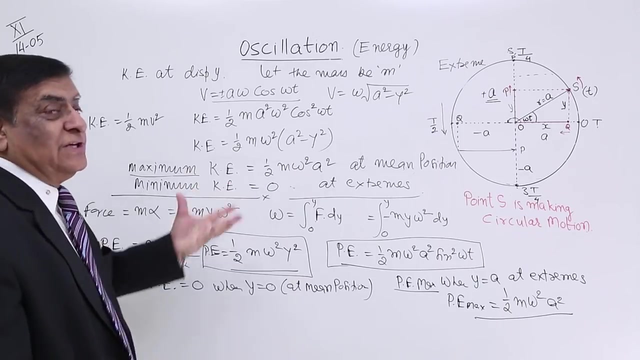 to y and t. these are maximum value and minimum value and their locations. where is potential energy? 0? 0 at mean position. What is kinetic energy at mean position? maximum, where potential energy is maximum at the extreme, and at the extreme kinetic energy is 0 and this is what we were seeing in case of a gravitational 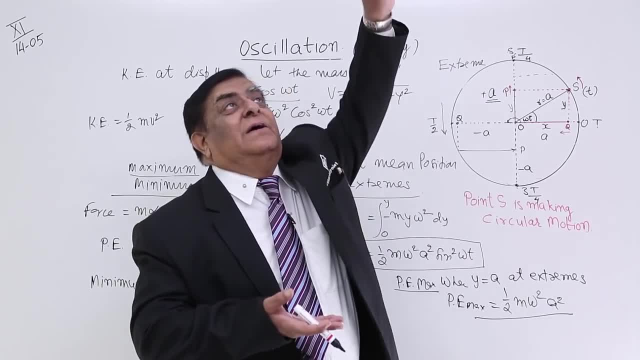 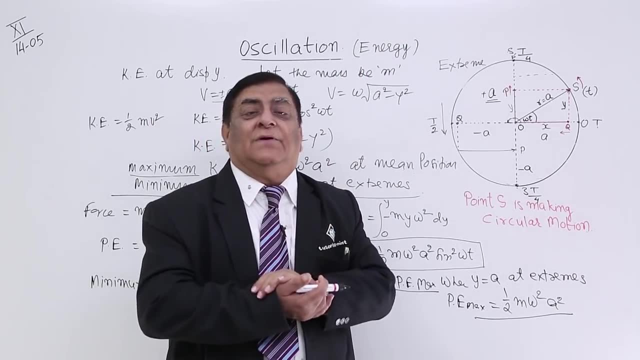 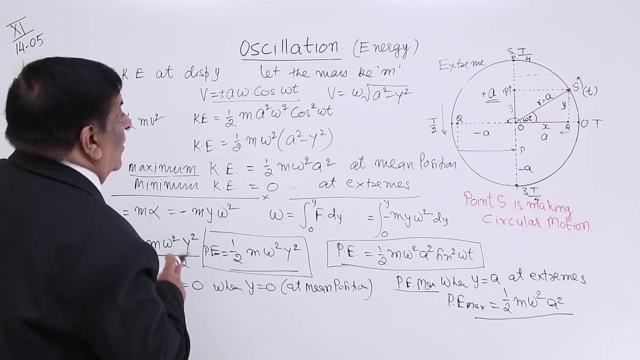 energy ball. here kinetic energy is maximum. here it is 0,. here potential energy is minimum. here potential energy is maximum, and their sum is always the same. is it the case here? Let us see the sum of two energies. the sum of two energies, how much is that? 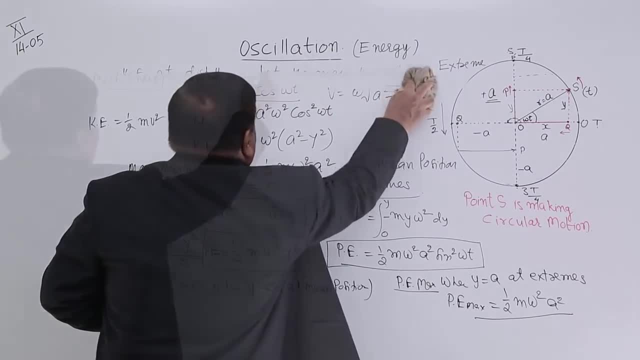 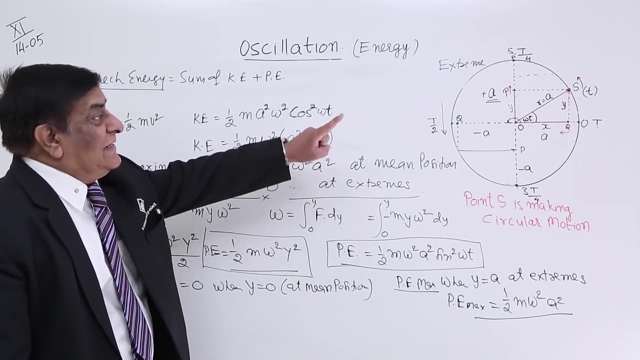 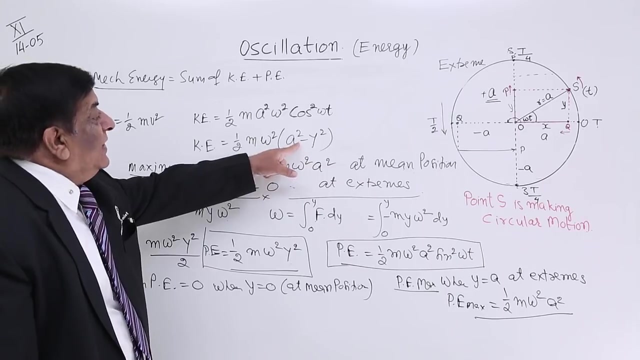 Let us see This sum we can make anywhere. let us say, at displacement y, this is potential energy and this is kinetic energy. add the two: half m, omega square is common, a is maximum. this is potential energy. Let us see the sum of two energies. the sum of two energies, how much is that? 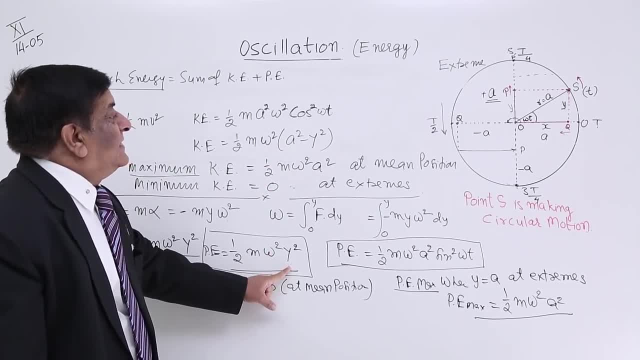 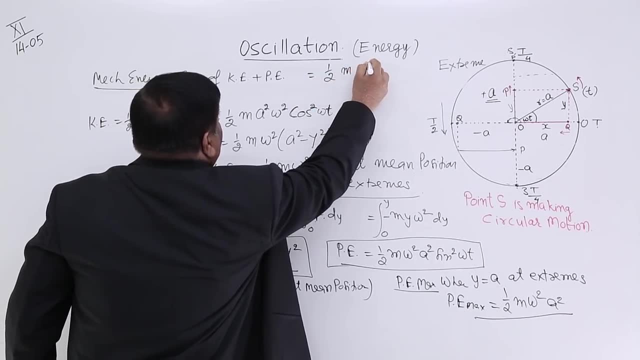 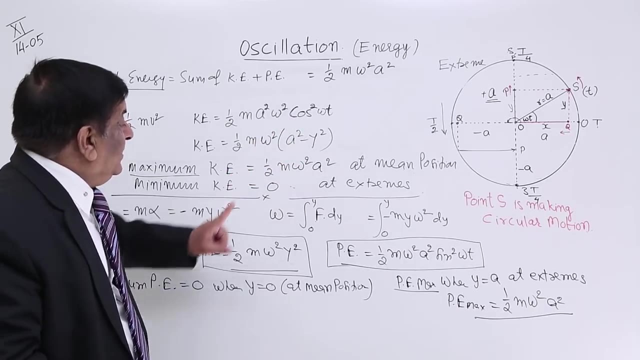 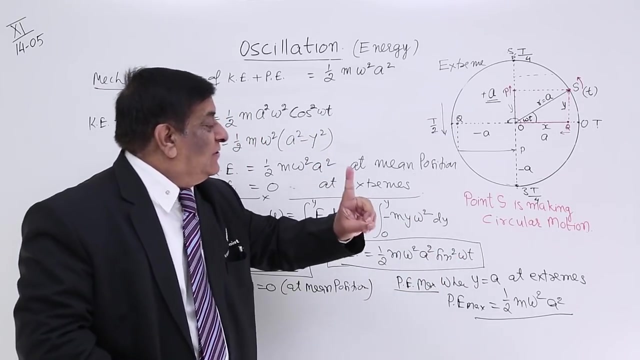 A square minus y. square plus y square is equal to only a square. so what do we get? Half m omega square. a square at time t. this kinetic energy at time t. this is potential energy. add the two cos square omega t plus sin square omega t is equal to 1, what is?